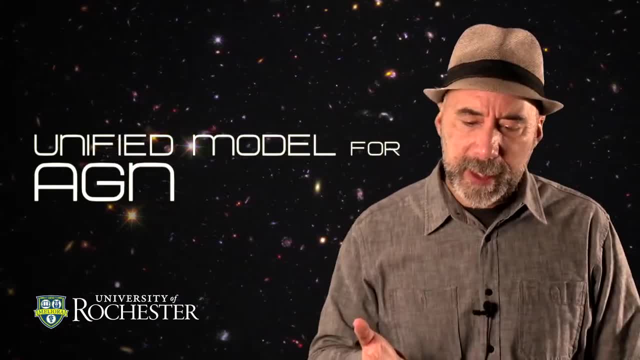 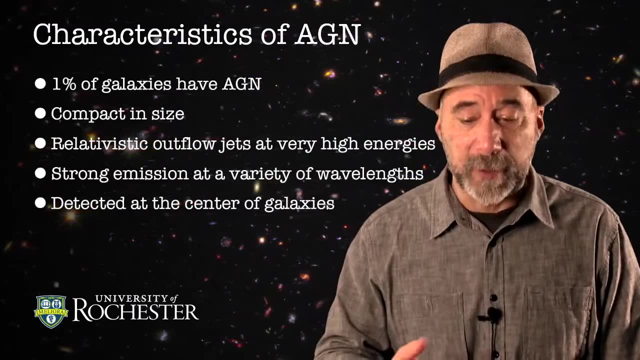 And that certainly has happened with active galactic nuclei. So the important thing to understand is: what are the sort of general characteristics of AGN? Well, they're compact in size. They tend to generate outflows at very high velocities, even the speed you know, close to the speed of light. So they're very relativistic. They 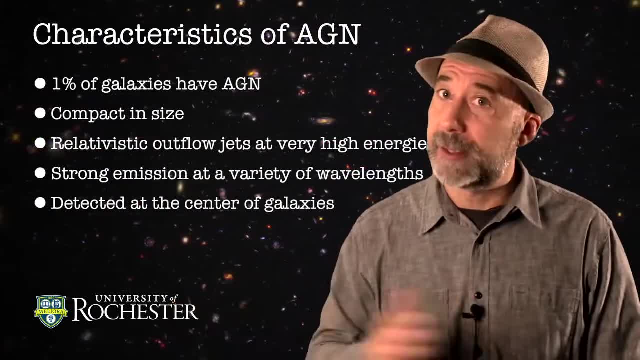 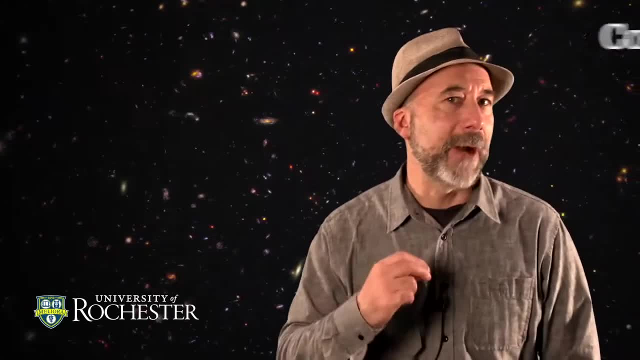 emit light at a variety of wavelengths. right, We've seen everything from radio to X-rays- And they tend to be at the center of galaxies. So out of this, people can back out certain unifying characteristics. Since the jets are relativistic, they tend to be at the center of galaxies. So out of 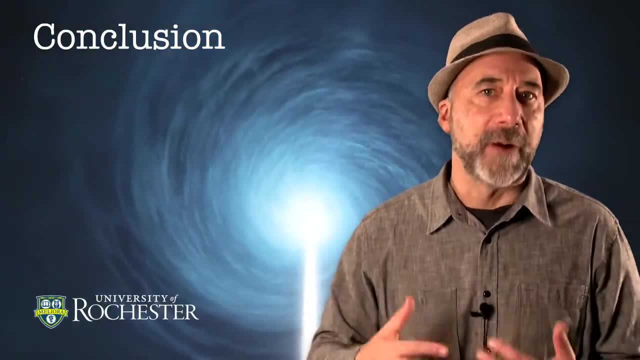 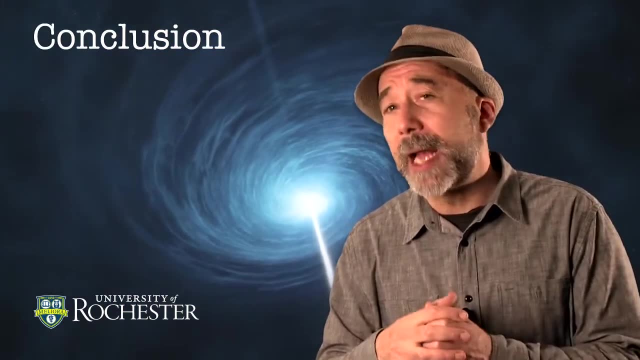 this, people can back out certain unifying characteristics. Since the jets are relativistic, the beams of gas are relativistic, they must be coming from something that is itself relativistic And that tells us and also the small size scale of these things. and one way we can. 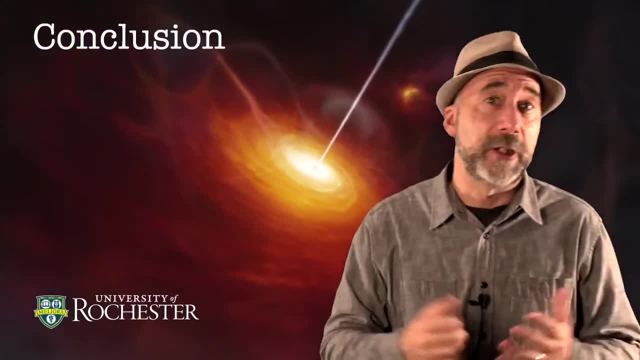 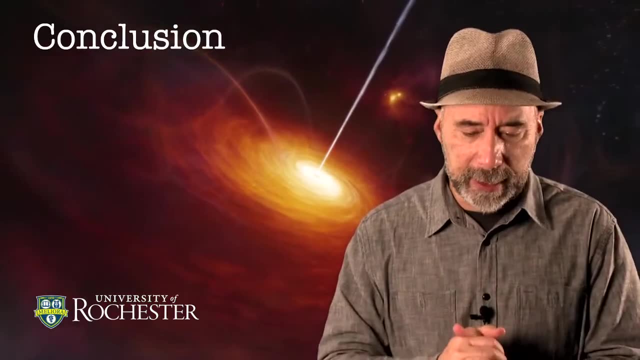 tell that they really are. the regions where these jets are coming from, or where all the energy is coming from, must be very small. is the variability, the fact that the variation sometimes is so fast that it must be associated with a small object. So you put that together. 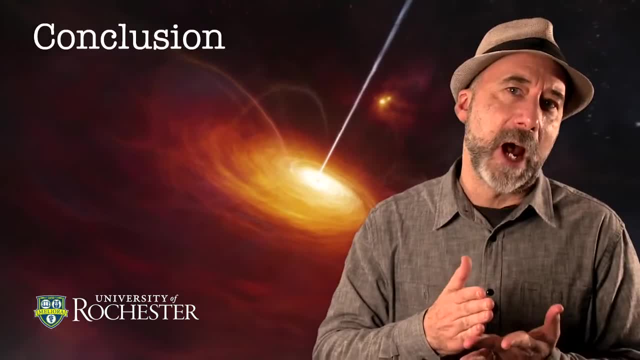 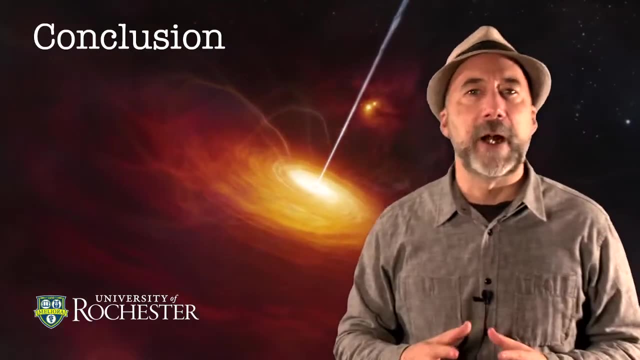 we got. we need something very small and we needed to boost things up to relativistic speeds. And that leads us to the idea that it's supermassive black holes, that it's black holes at the center of these galaxies, just like, you know, at the center of our own galaxy, that that's. 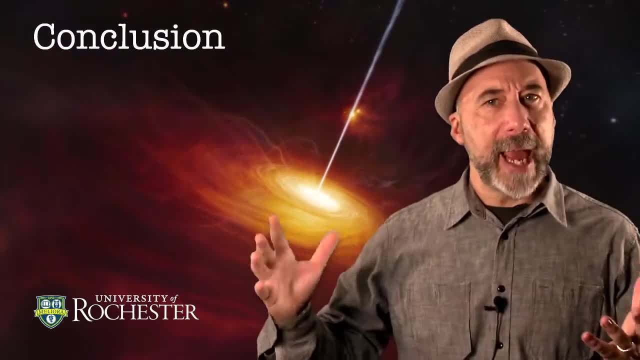 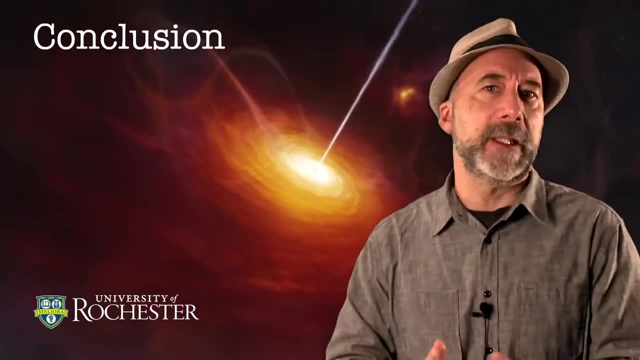 really the engine powering active galactic nuclei. So, as gas falls inward towards the black hole, if there's gas available, then it's going to be, as we've talked about before: the friction between the materials, the tidal forces that as it falls in, of course, before it gets to the event horizon, that's where the energy. 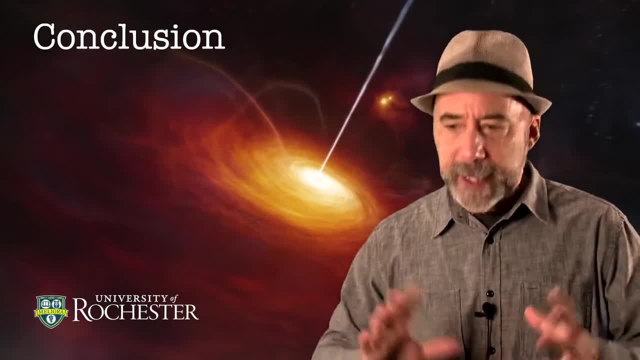 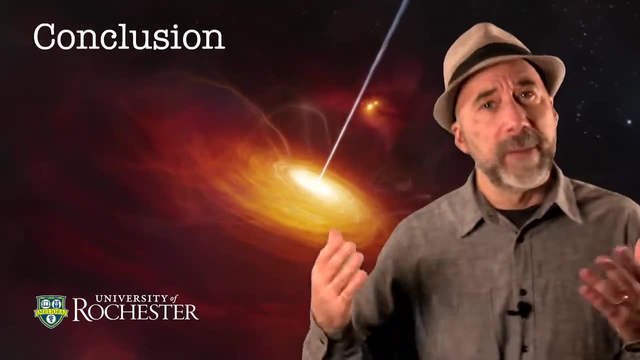 is going to be coming from And the jets that we see are coming from the accretion disk of material that forms as material spirals in towards the black hole, And we've already seen how jets can form from accretion disks when we looked at young stellar. 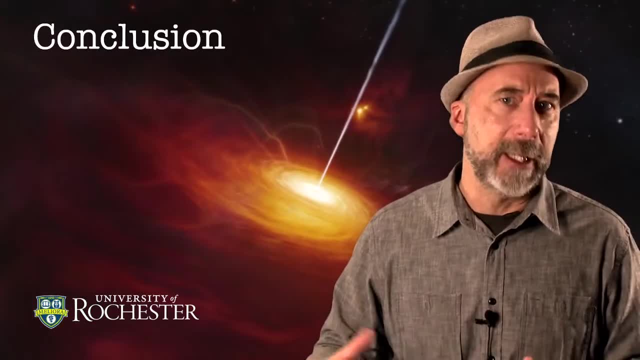 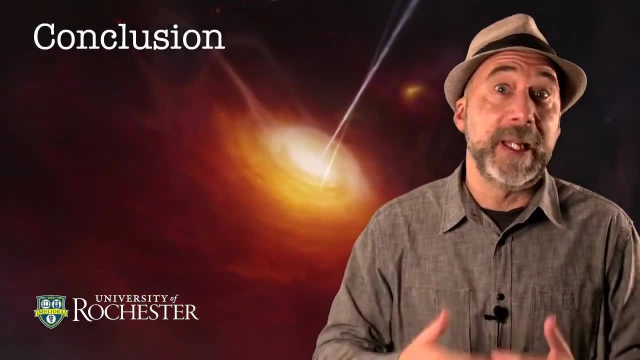 objects. So anytime you form an accretion disk, you're likely to get a jet forming. In this case, because it's close to a black hole and you need to escape from the regions close to a black hole, the speeds are naturally going to be close to the escape speed, which 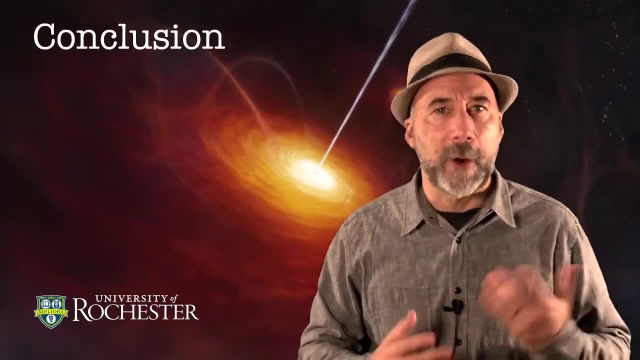 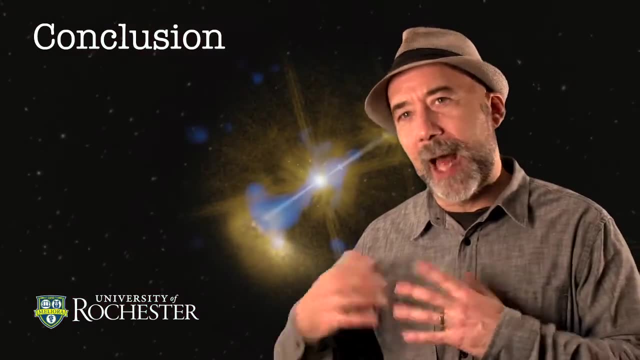 is going to be close to the speed of light. So you know, supermassive black holes are really at the root of the AGN phenomena, the active galactic nuclei phenomena, And the reason why every galaxy doesn't have an active galactic nuclei is because it's 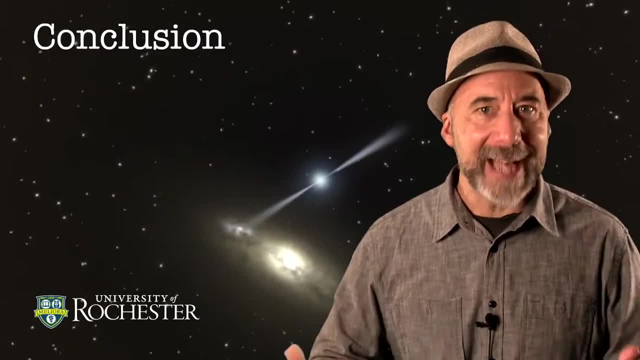 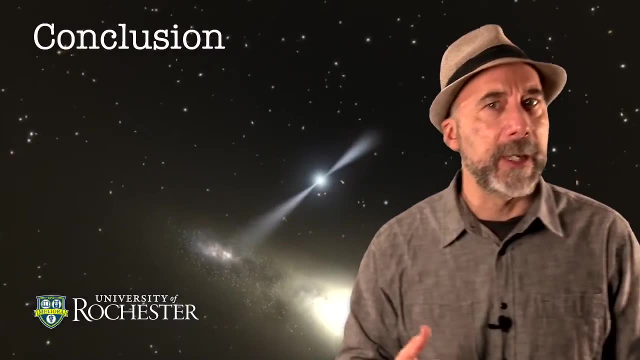 just a matter of whether or not there's enough mass there. There has to be a lot of gas available to funnel into the black hole in order to produce the kinds of emission that we see. So, really, what we're also learning about here is the fact that, as galaxies evolve, we expect 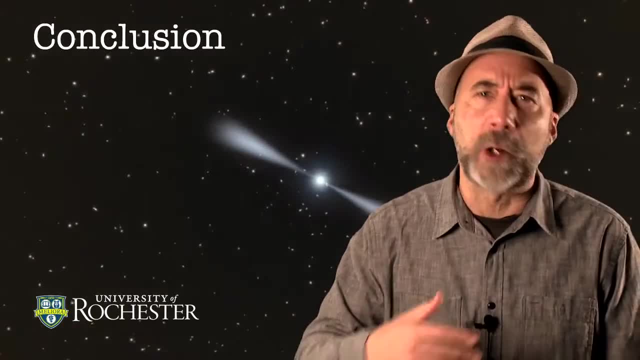 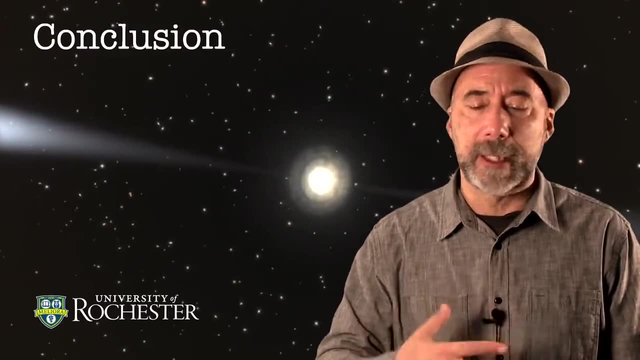 that perhaps they will all go through a quasar-like phase, an active galactic, nuclei-like phase, But once they run out of material in the central regions, as has happened in our own galaxy, then they quiet down. So how does this help us tell the difference between all of the different kinds of active? 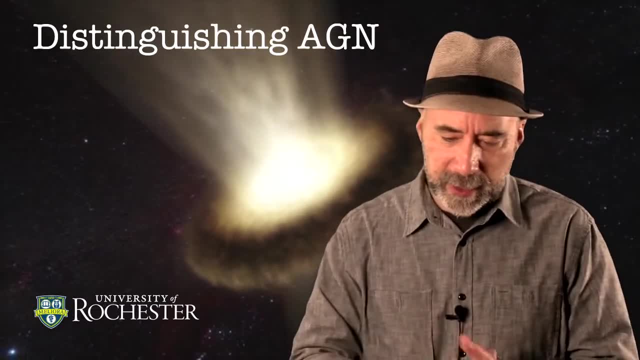 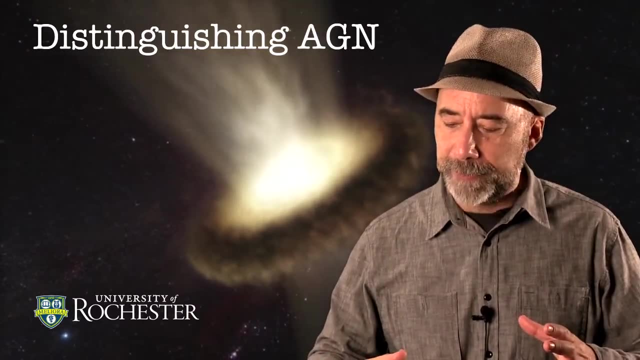 galactic nuclei. Remember we had the radio galaxies, the quasars, the seafords, etc. And it really turns all out to be orientation. So what we imagine is that we have, you know, a central black hole and then we have a disk. 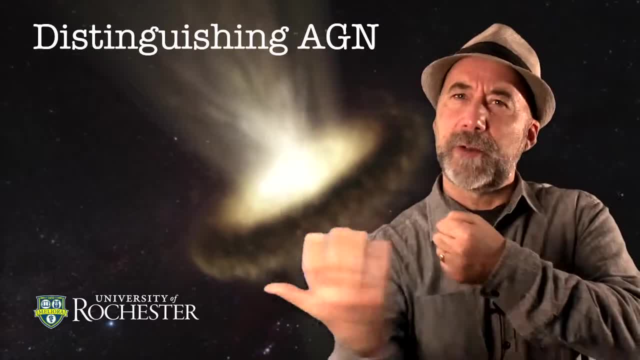 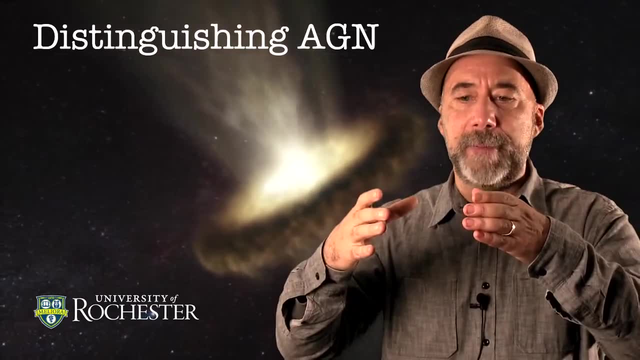 around it And then around that, people have hypothesized that there's actually sort of a ring of molecular gas And that's actually sort of you know, sort of quite that. Now what matters is whether or not that ring is tilted towards you or perpendicular to. your line of sight, And if it's perpendicular to the line of sight, then you're not going to be able to see through it. You may not see some of the central regions, but you will see the jets beaming up on the plane of the sky. 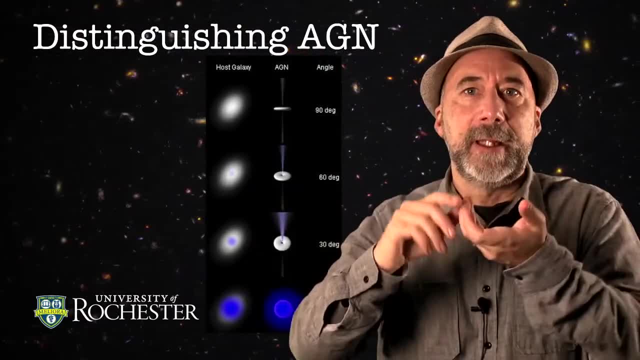 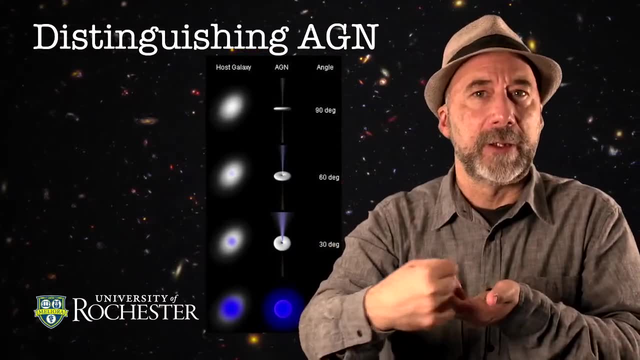 However, if the entire system is tilted right at you, then the jet is going to be coming right at you And you won't necessarily see the jet directly, but you will be able to peer right down into the center of the whole region. 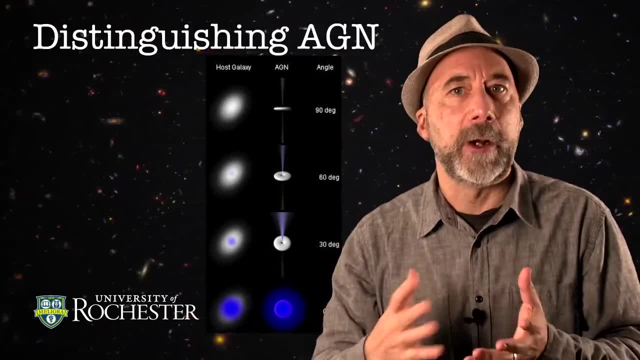 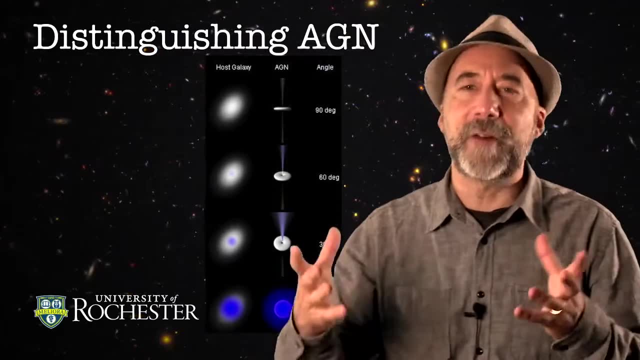 Or the center of the whole system, And so you know, you're going to see a lot more energetic phenomena as well. So really it turns out that with just these unifying, this unifying model of a torus, a molecular torus, an accretion disk and a supermassive black hole, we're able to actually 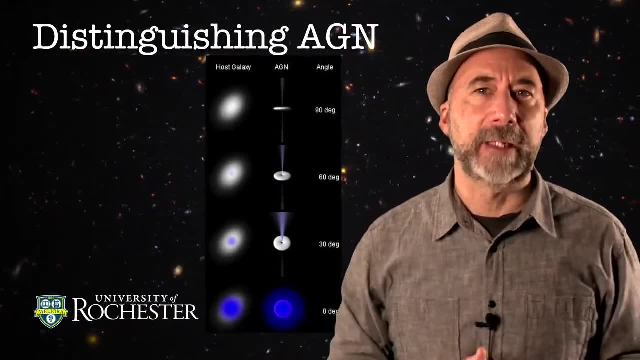 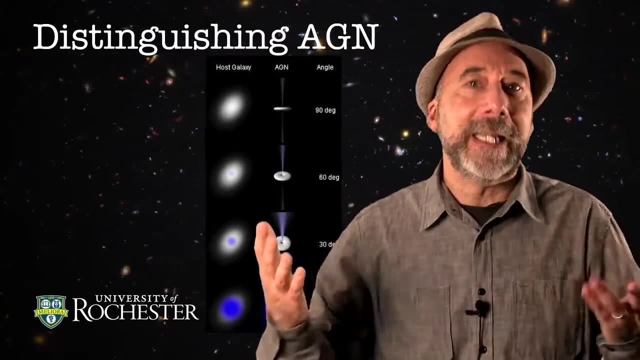 embrace all of the phenomena, all of the different types of active galactic nuclei, And when you come up with something like that as a scientist, you get really excited because you found simplicity in complexity, And that's what every scientist is looking for. 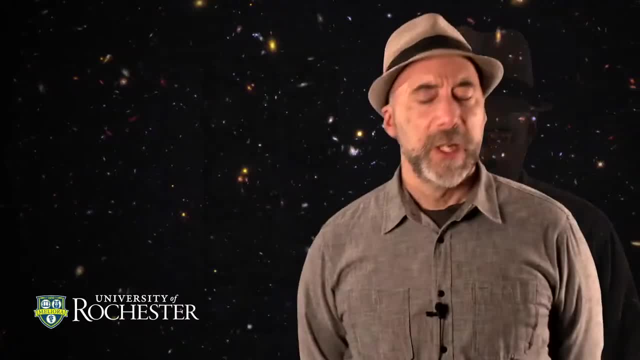 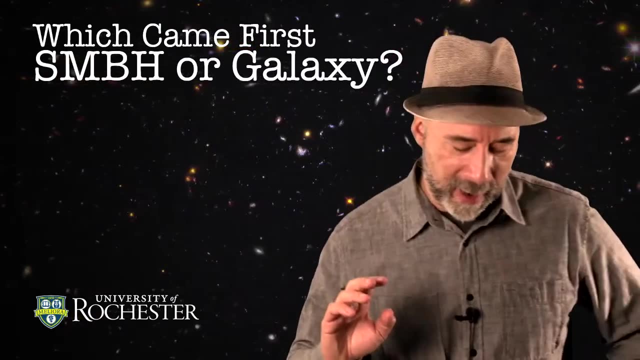 Whether they're biologists, sociologists or physicists. So now that we've seen that, you know, supermassive black holes occur in all galaxies and that they are responsible for the amazing active galactic nuclei phenomena, we can ask the